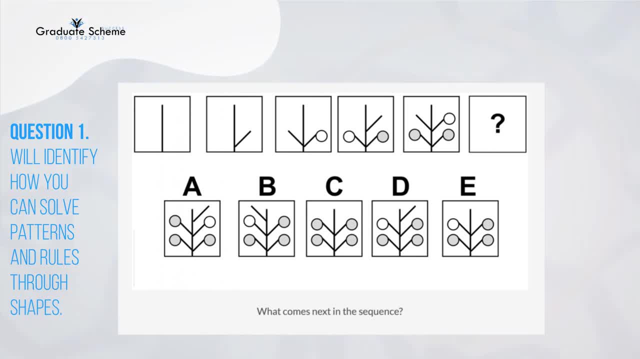 Out of the options shown to you, it may first appear that the answers are all very similar. If you struggle to find the correct answer, you can use the Q&A box in theathnet to find the answers to your questions and test the questions in the following steps. 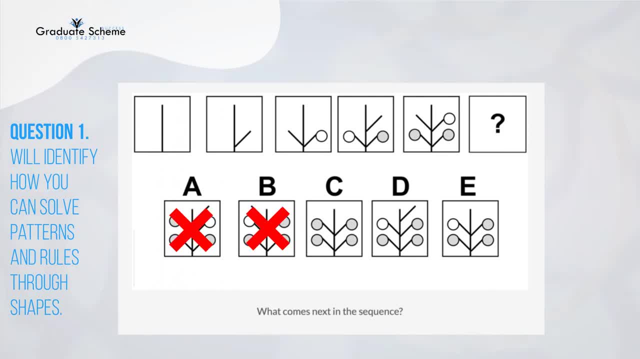 find the correct answer. use a process of elimination to eradicate any possible solutions or non-possible solutions. as shown here, The correct answer here is D. This is because the white ball moves across on the same level and a new branch is created on the right, where it always. 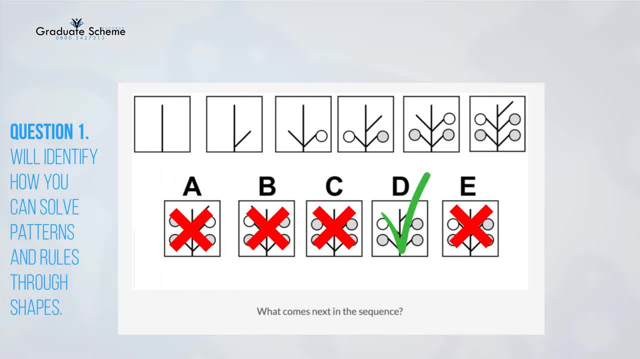 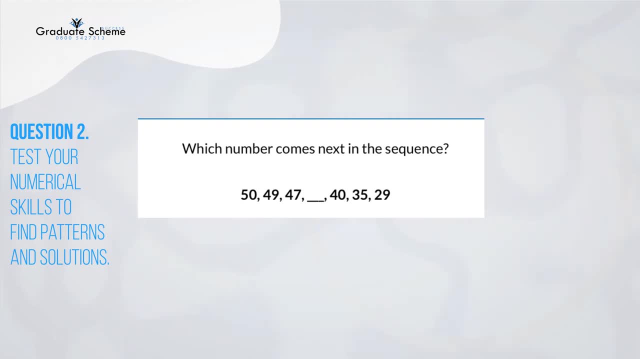 starts first. Question two: Another type of question you may expect in a logical reasoning test may be to test your numerical skills to find patterns and solutions. So, as we can see here, which number comes next in this sequence? 50,, 49,, 47, blank, 40, 35 and 29.. As the missing: 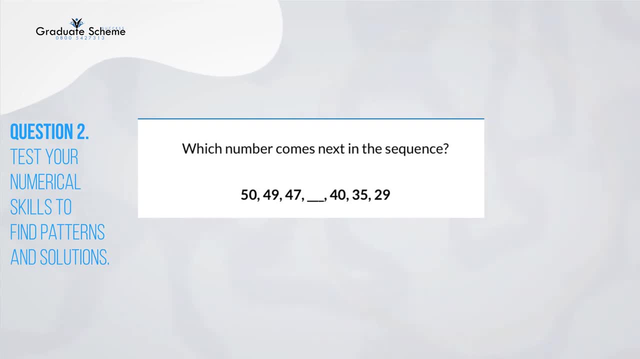 number is in the middle of the equation. the correct answer is D. In the middle of this sequence, we can work both forwards and backwards to identify the pattern. Firstly, let's look at the potential answers that are given to you In this question. we know that this will be in the range of 41 to 46.. 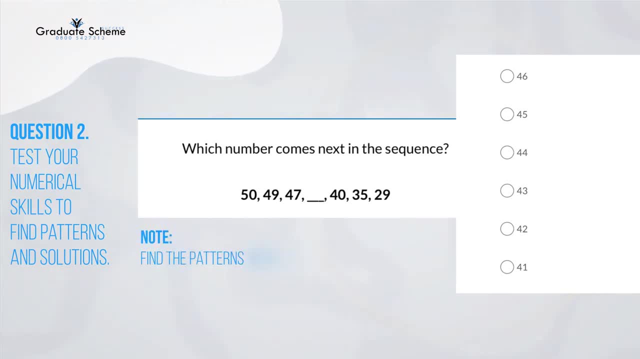 To approach this question, first find the pattern with the first three numbers With some basic mathematical skills. here there is a pattern of subtraction, distribution and multiplication. So let's look at the pattern with the first three numbers. For example, we go from 50 to 49 minus 1.. 49 to 47 minus 2.. So we would expect 47 to go minus 3 to 48. 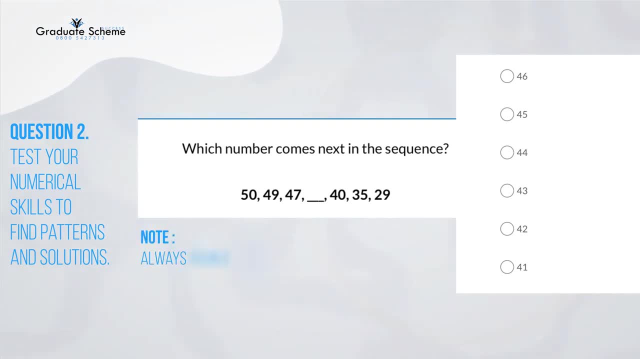 However, it's worth double checking. Moving upwards, we can see: 29 to 35 is 6.. 35 to 4 is 6.. For 40, the difference is 5.. 40 to 44, we would expect 4.. So for both ways this pattern fits. 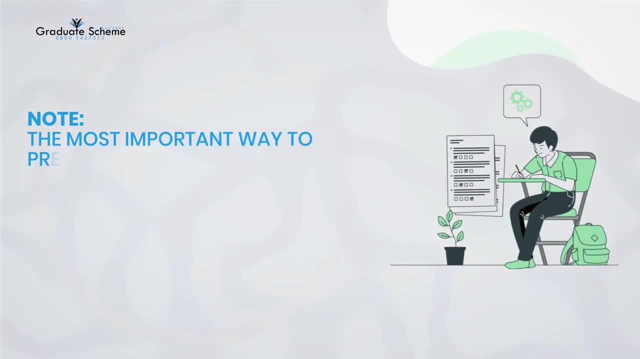 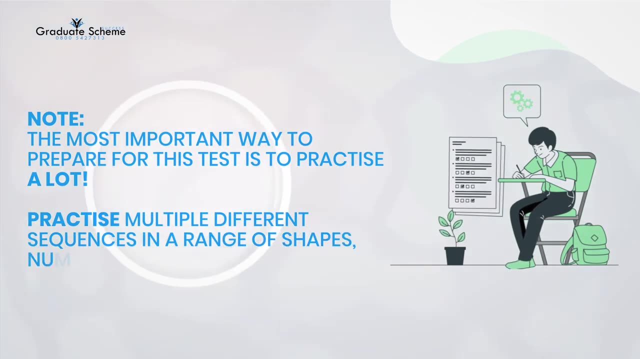 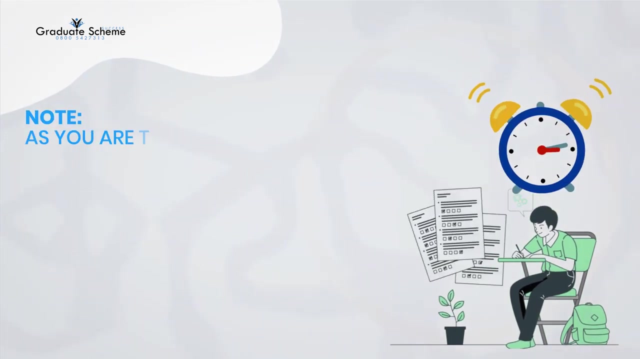 The most important way to prepare for these tests is to practice, Practice multiple different sequences in a range of shapes, numbers and patterns that can provide you with the support and guidance that you need. As you are time, you will need to practice multiple different sequences. 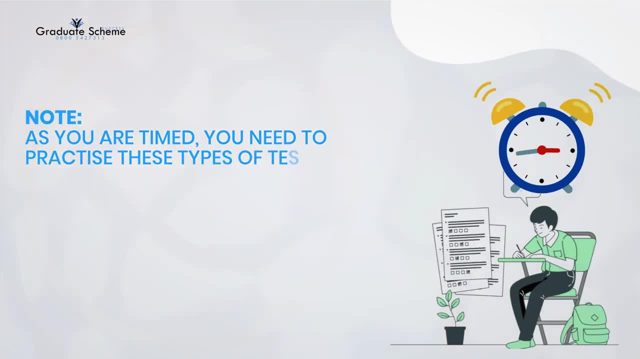 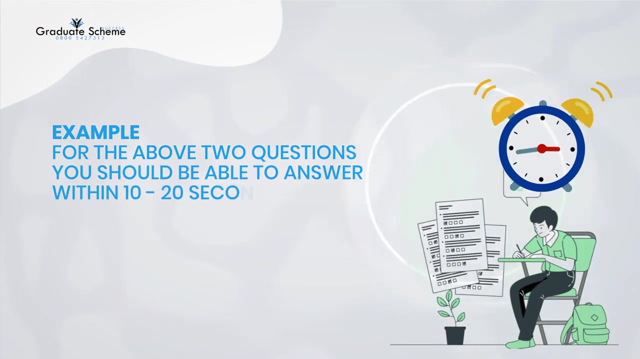 You need to practice these types of tests within a set time limit. The quicker you can do these tests, the better. For example, for the above two, you should be able to answer each of them within a time period of between 10 and 20 seconds. Finally, I would urge you to use the support that 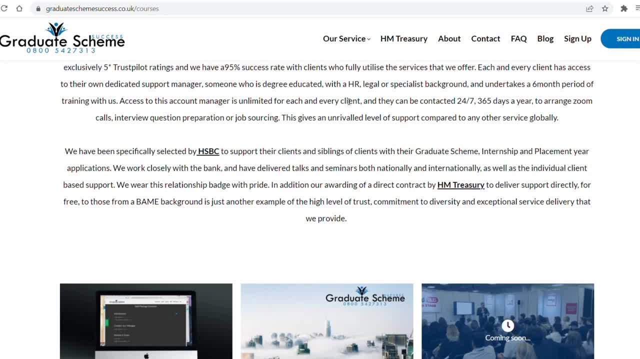 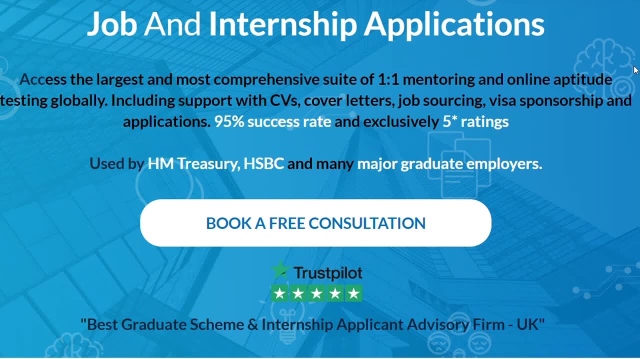 we have available the free practice support at graduateschemessuccesscouk, Or book a free consultation so we can show you how we support with these types of testing.